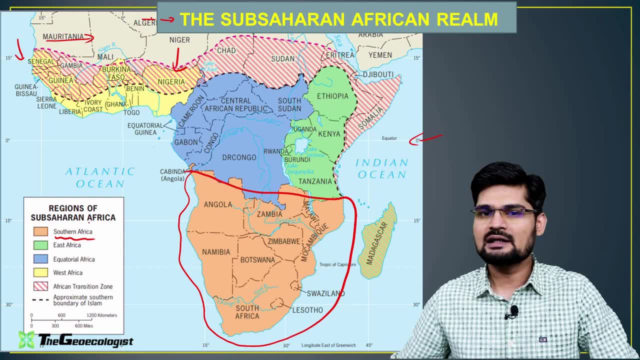 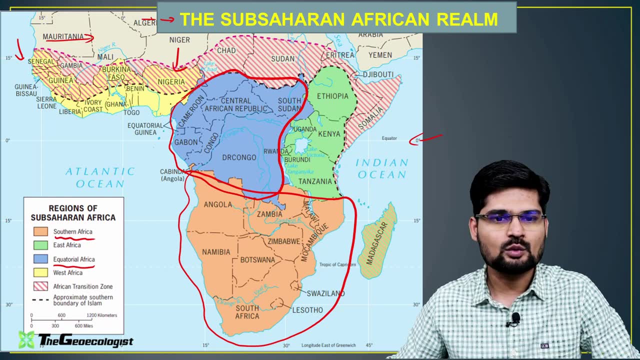 here is the Southern African region that we'll be learning today. Then in between you have the Equatorial Africa. If you observe this region is Equatorial Africa, Then we'll also be looking into the West African countries, this coastal countries on West Africa, and also we'll be learning about. 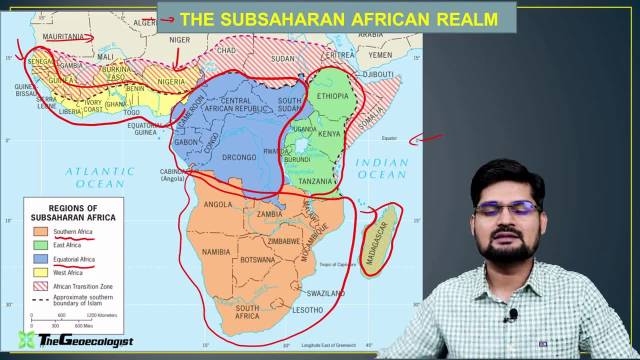 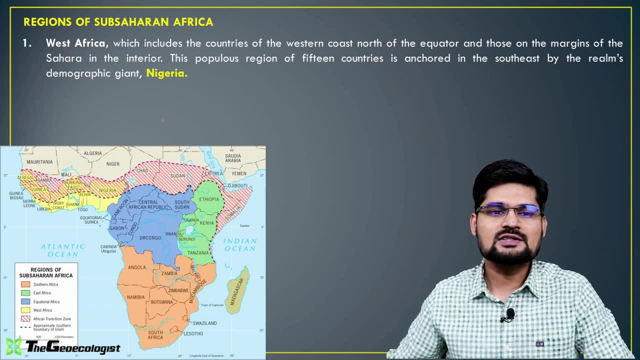 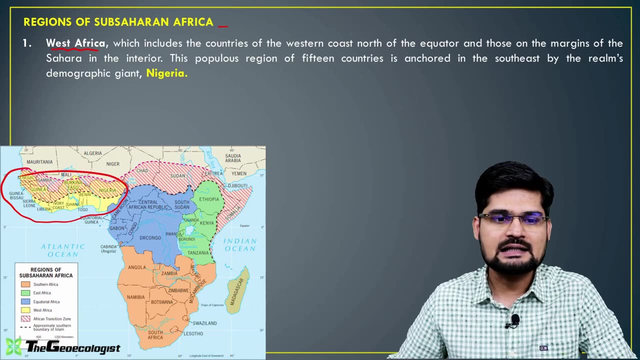 the East African countries, including the Madagascar. So now let's divide the sub-Saharan African realm into these regions and understand their configuration. So, regions of sub-Saharan Africa: the first one, as you know, is the West African region, This particular West African region, if you observe, and Nigeria is the most dominant country in this. 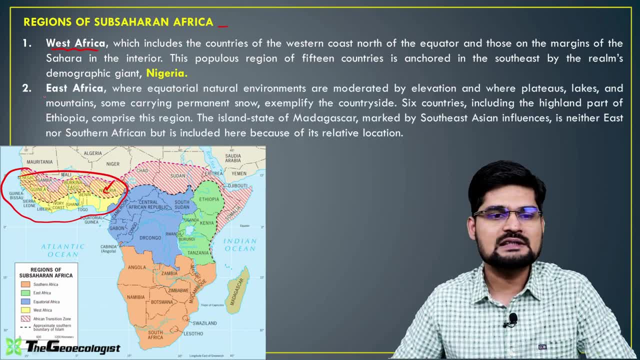 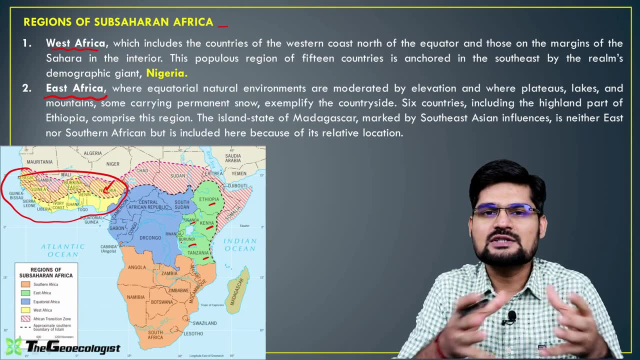 particular region, So we'll be looking into it Then further, if you observe the East African region Here you observe Ethiopia, Kenya, Uganda, Burundi and Tanzania. These countries are majorly part of East Africa, and also we'll be including Madagascar in our learning as well. Then let's 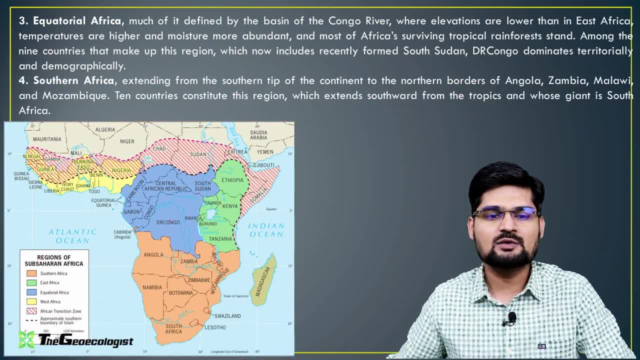 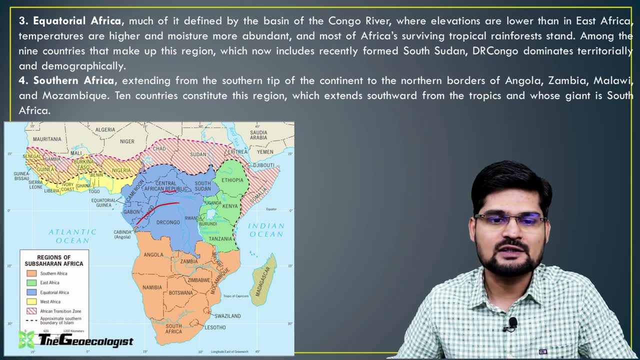 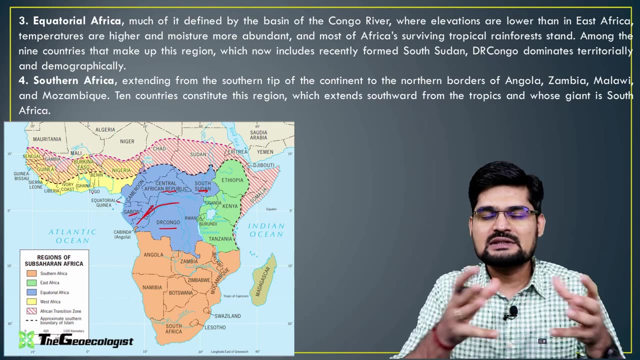 understand the Equatorial Africa, and this is majorly drained by the Congo River, if you remember- and earlier it was also called Zaire, and the countries here are Central African Republic, South Sudan, DR Congo, that is, Democratic Republic of Congo, Then you have Congo, Gabon and Equatorial Guinea. So these are the areas and then we'll be going to. 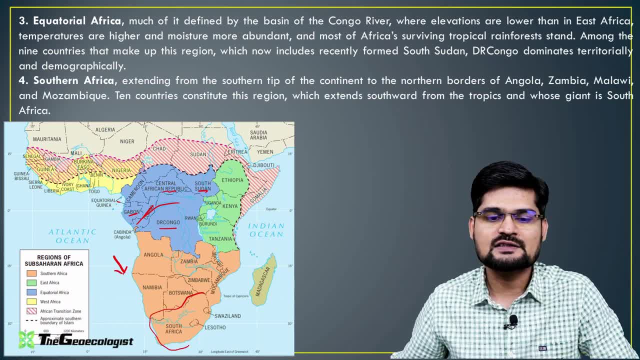 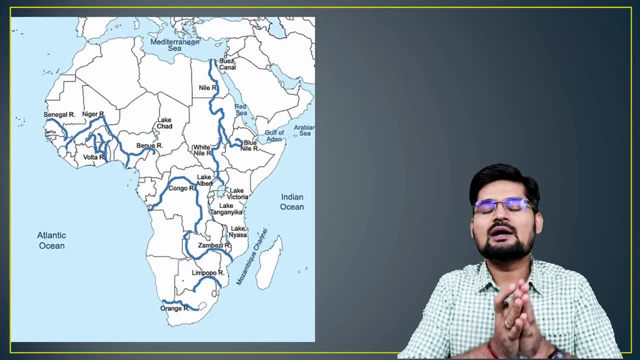 the Southern Africa, where South Africa itself is the biggest country and the most famous country across the world. So we'll be learning about this Southern African region. So now, first thing that we need to look into is the river system of African continent. So if you observe Nile River and its 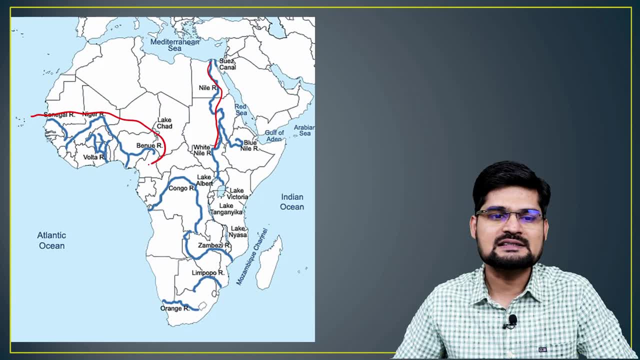 major river in the West African segment is the River Senegal out here and River Niger out here, and then also we have River Volta and Benue out here and you have Lake Chad. Then if you go down south out here, the Nile is divided into White and Blue Nile, if you remember carefully. So Blue Nile. 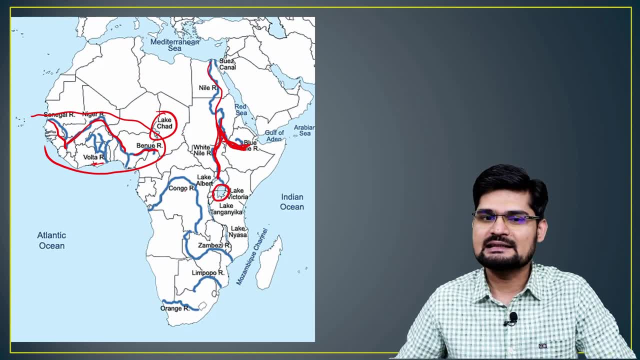 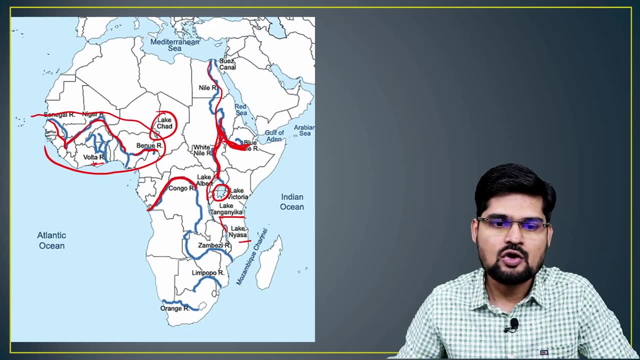 and White Nile right from Lake Victoria. it is connected in Tanzania, Lake Albert, then you have Lake Tanganyika, then you have Lake Nyasa and here is the biggest river in the West African segment. Then you have the River Congo River system- if you observe here- and then you have the Zambezi River. 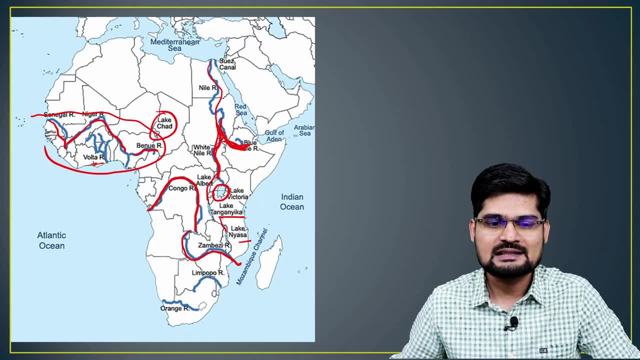 system down south, and also one important river, that is, Limpopo River, which is like a boundary between the South Africa and adjoining country Botswana, and here you have the Orange River, the most famous river of South Africa. So these are the major river and, if you observe, Atlantic. 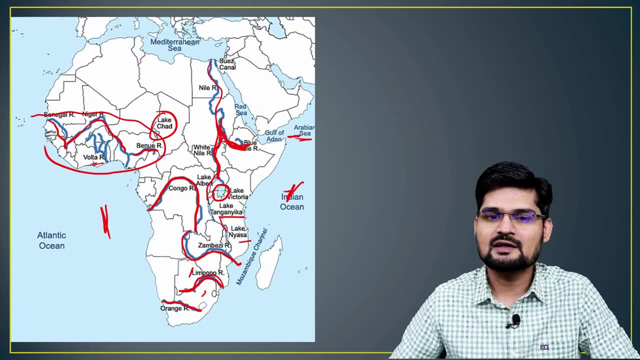 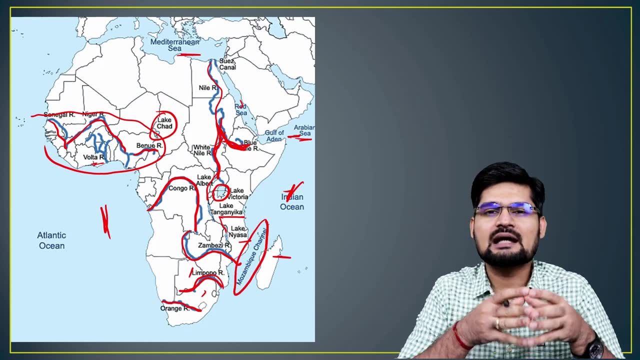 Ocean here. then you have Indian Ocean here Gulf of Aden, Arabian Sea here, Red Sea here North Mediterranean, and then you have the Mozambique Channel which separates the Madagascar- and it's alongside the islands- with the mainland Africa. So this is the water. 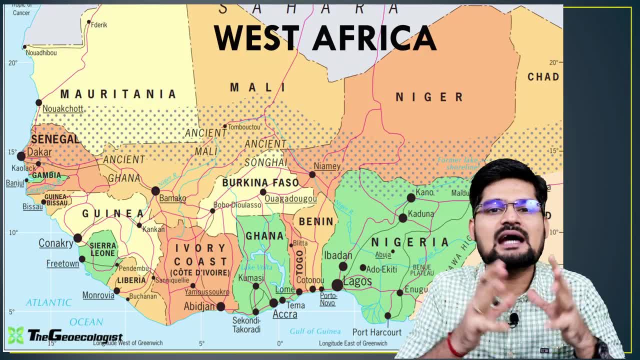 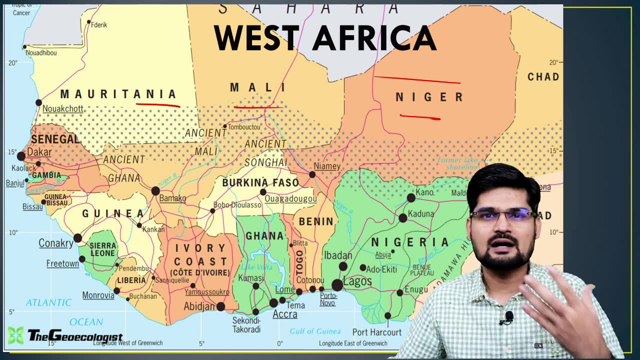 bodies. if you carefully see, Then let's look into the West African region first now. So if you carefully observe these, Mauritiana, Mali and Niger are the major areas of the Sahara desert, and then you come to Sub-Saharan Africa. So if you observe Nigeria out here, Adamawa Highlands out, 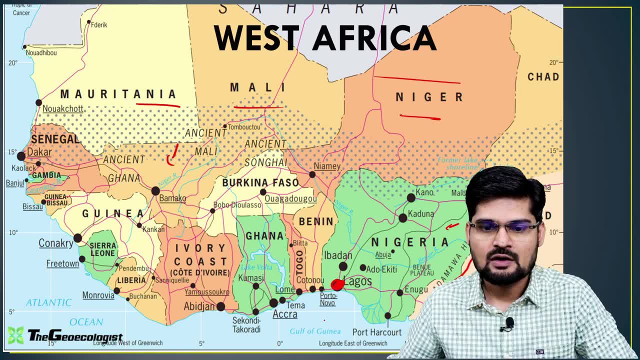 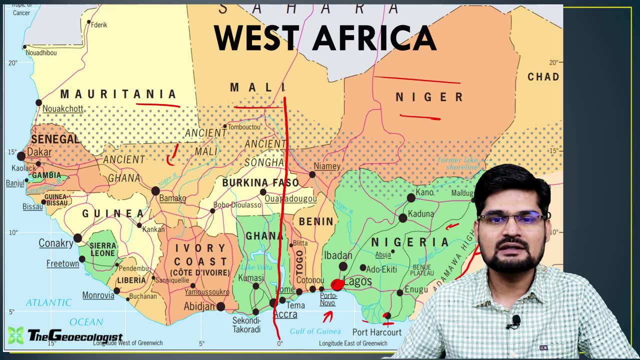 here, and then you have the capital of Nigeria, Lagos, in the Gulf of Guinea, and then you have Harcourt out here. So this is important: The zero-degree meridian that we have already learned. this is the green, which meantime zero-degree meridian passes through these countries. 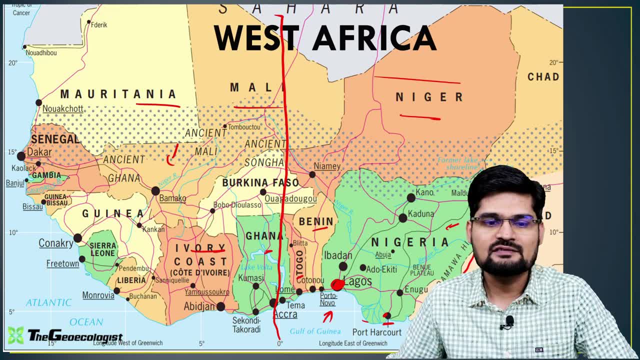 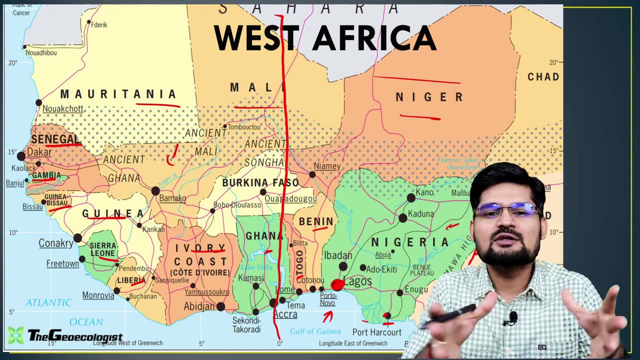 So you have Ghana, then you have Benin, then you have Togo out here, Ivory Coast, Liberia, Sierra Leone, Guinea and Guinea Bissau. then you have Gambia, Senegal. All these countries are located in the Western Africa. Now, by far, if you observe, Nigeria is the biggest country, and we are going to 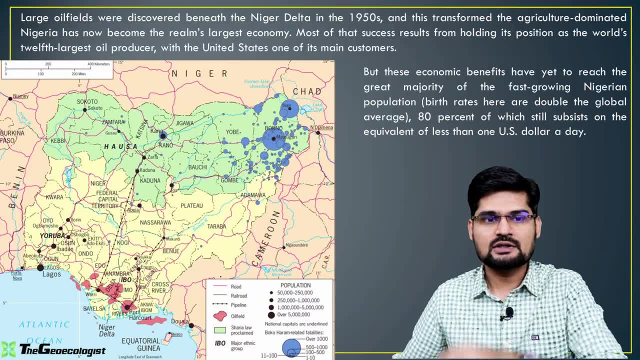 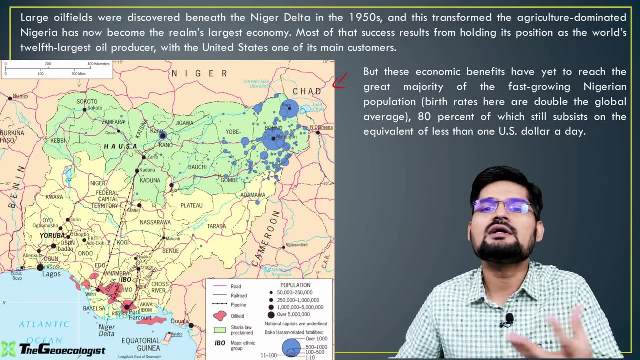 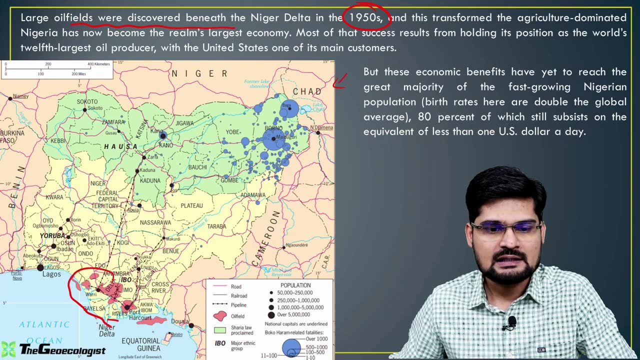 look into further details around these countries. So look here, the first thing that we talk about is the country Nigeria. So Nigeria has recently been part of the world oil trade and large oil fields were discovered in 1950s near this delta area. If you observe this red zones out here, these are the 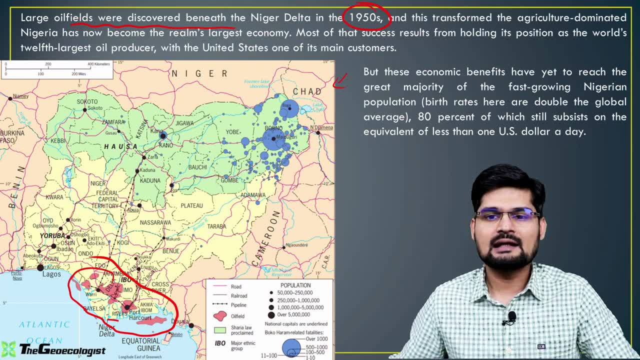 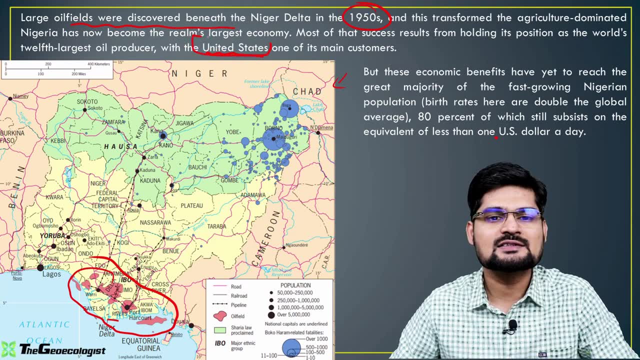 oil fields which are the major source of economy in Nigeria and economic benefits have increased gradually and Nigeria has the major oil supply to United States, So United States is its main customer. that we observe The Northern Nigeria. if you observe this green patch out, here is also. 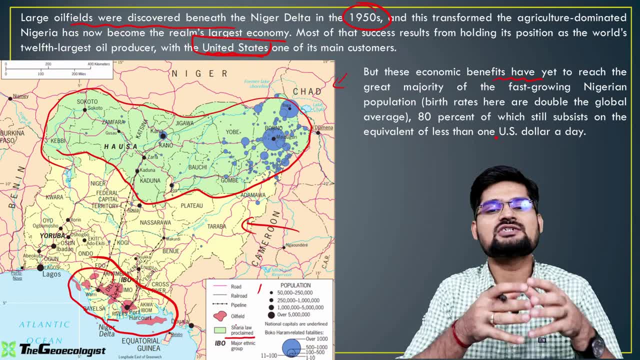 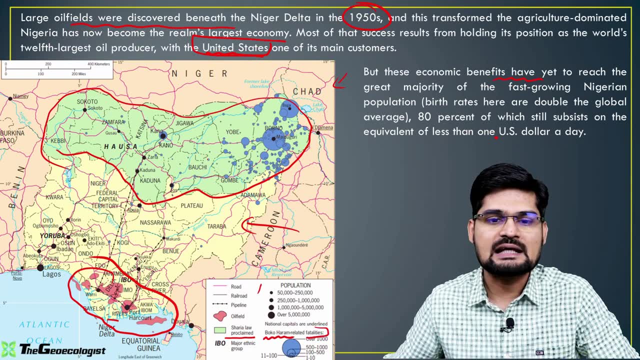 dominated by the Sharia government. that is the Sharia law. It is governed through the Islamic Republic and then, if you observe carefully, you have the Boko Haram related fatalities in this northeastern region, the Borno and adjoining areas. Boko Haram is one of the terrorist organizations. 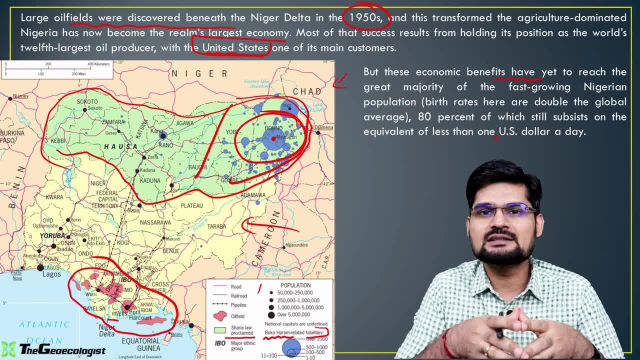 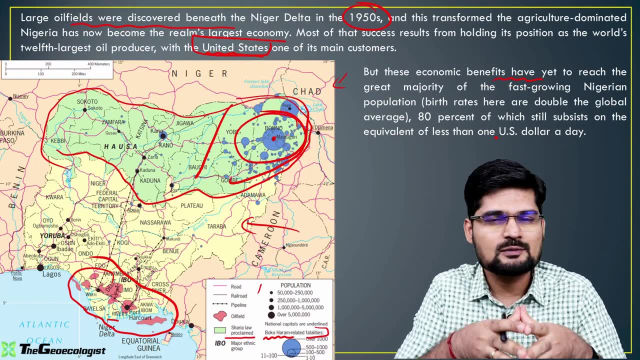 we say who is opposing the West Western culture? and they want their own traditional culture out there and they have given arms and hands of children as well. So a lot of news about Boko Haram is always there. So this is a tormentor. So let's look into the regional area of Nigeria and the advantages of this region. 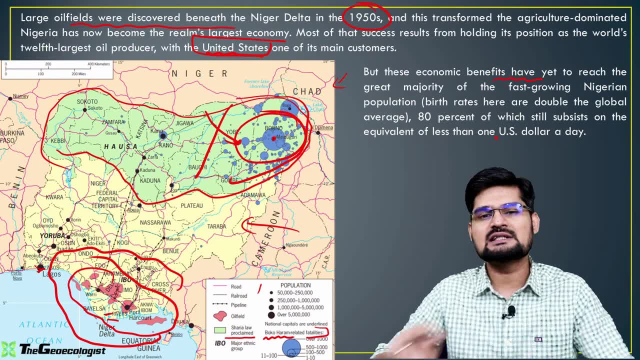 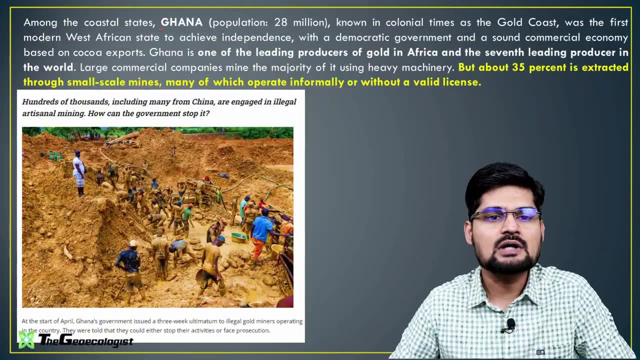 We have the places we call Ghana. Ghana is the most property in Nigeria. It is the most thing that people understand about this region from this point of view, so that people who talk about Ghana they are getting used to this region. So theana, that is the most important. 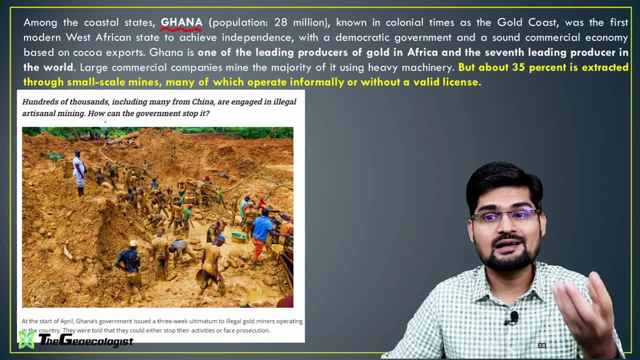 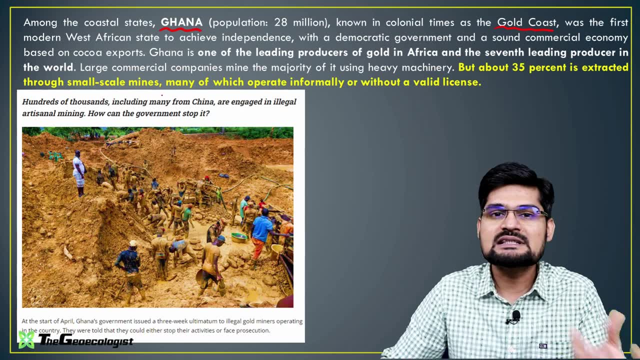 place to live in Nigeria. So now let's look into the coastal area of the south, the most popular and most important place around here, which is called Ghana. If you observe, this is in the northern deltas of Nigeria- it is the most prosperous and most represented belt of Nigeria. 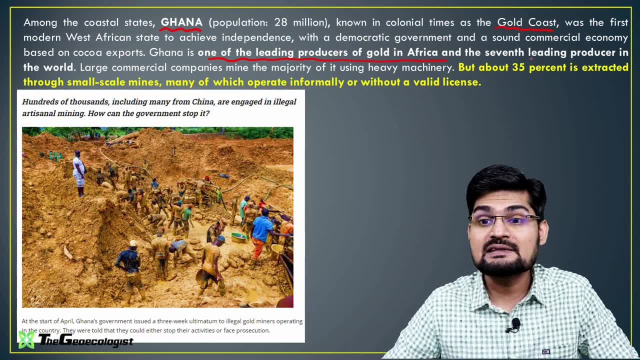 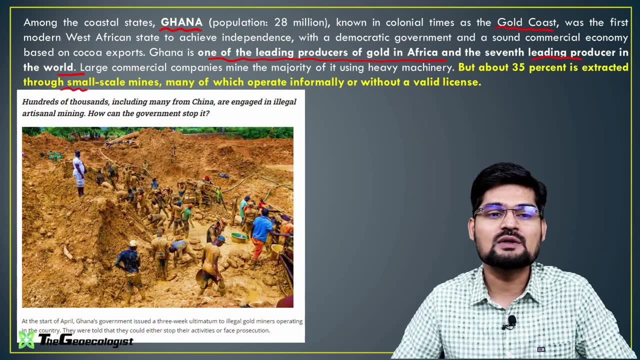 So Ghana is one of the leading producers of gold in Africa, seventh leading producer in the world. But then there is a question: why is it so poor? So remember, 35% of the gold is extracted through small mining and also informally operated. 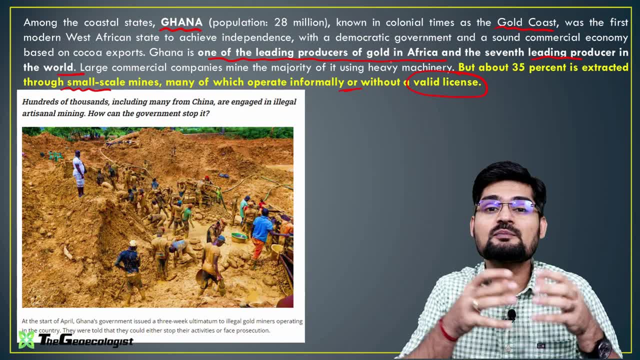 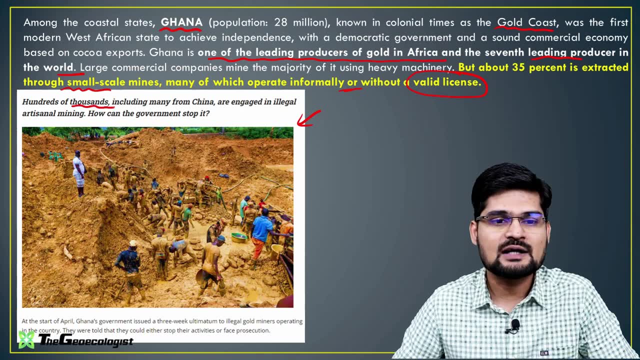 and also without, many times, a valid license. So a lot of problems in terms of mining is there And remember, this kind of news is very common in picture. Hundreds of thousands, including many from China, are engaged in illegal artisanal mining. 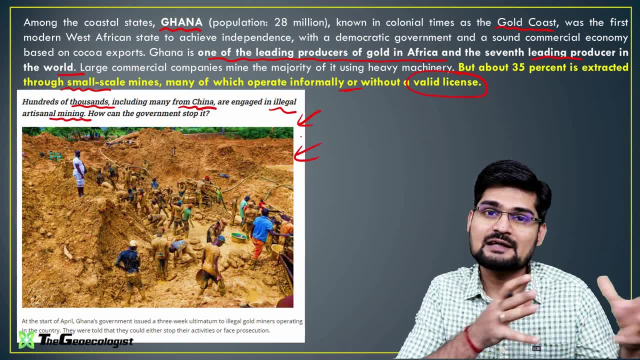 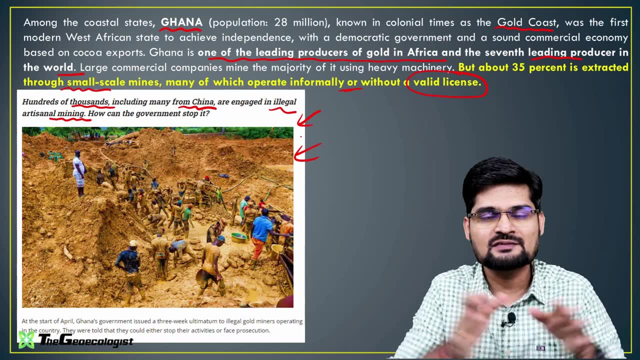 Remember, these are the placer deposits, placer gold deposits, like Brazilian highlands, Ghana also has, because their timing of formation was same. a jigsaw fit continental hypothesis, If you observe the theory that says that once they were part of the same formation. so the 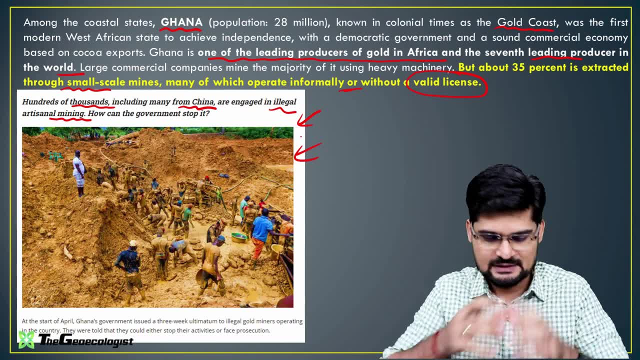 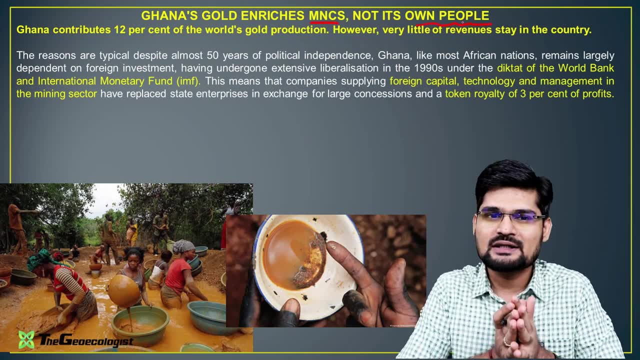 gold is available in large quantities out here in the placer deposits And, if you observe, Ghana's gold enriches MNCs, not its own people. This is very commonly in news And this is one important theory that you need to look into is resource curse theory. 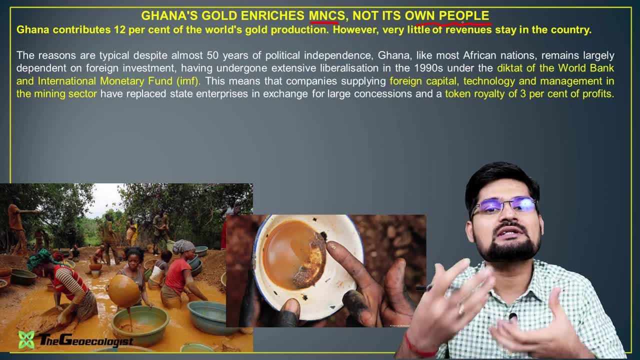 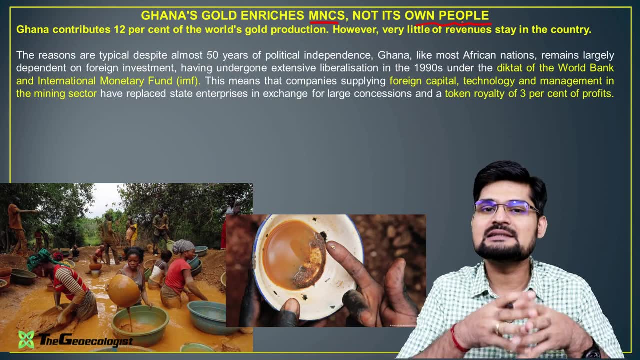 What does it say? That this country do not have enough human resource to exploit their own natural resources. Hence people coming from outside multinational corporations. they help these people to drain out the country's wealth And in order to drain, they give the token royalty of just 3%. 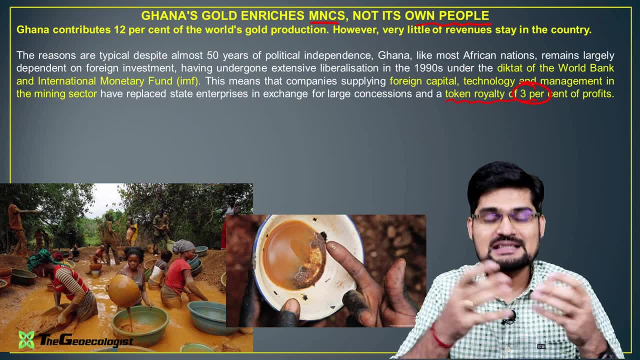 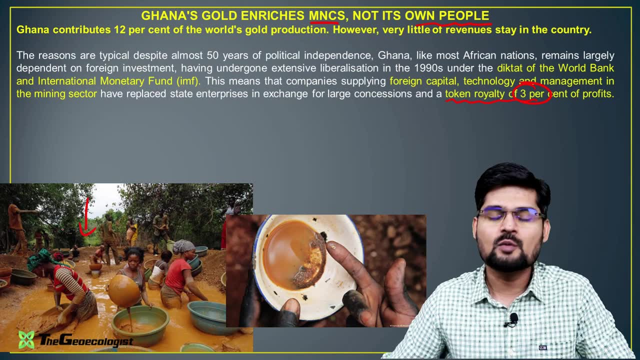 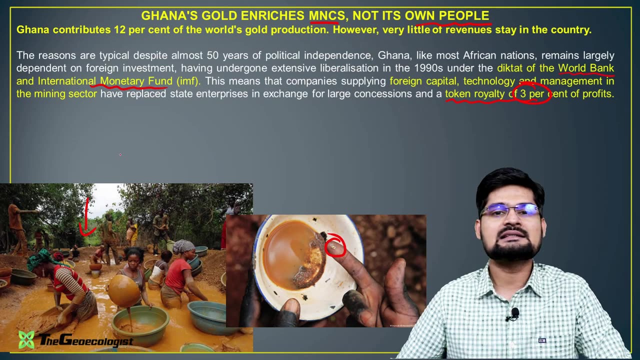 And they also take away the wealth in the name of helping. So this is something which is very interesting, And Ghana is not benefiting by its own resources. So if you observe this kind of open mining happening, this kind of gold traces, Placer deposits right International Monetary Fund and World Bank Tic Tacs, the liberalization. 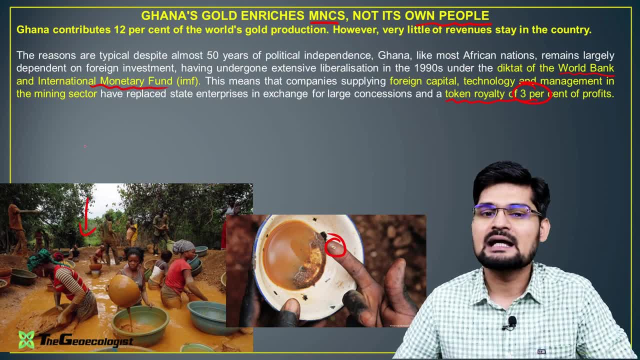 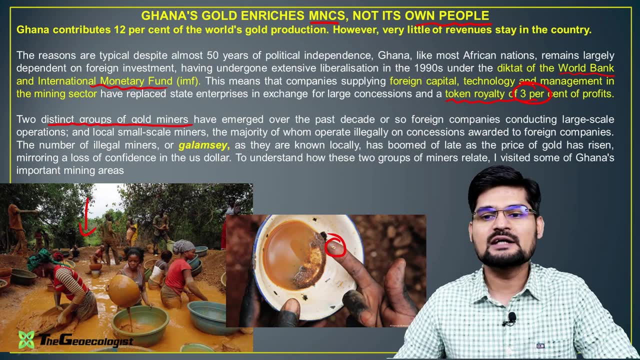 of Ghana's economy and intervention of the multinationals, And that is what is taking away the resources out. So, if you observe, there are two distinct groups of gold miners out here, And one of them, which is conducting illegal mining, is called gallancy. 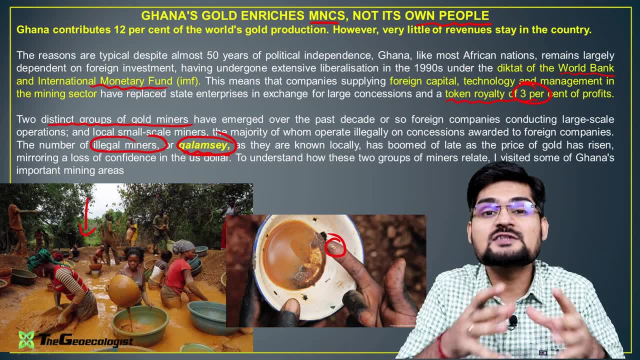 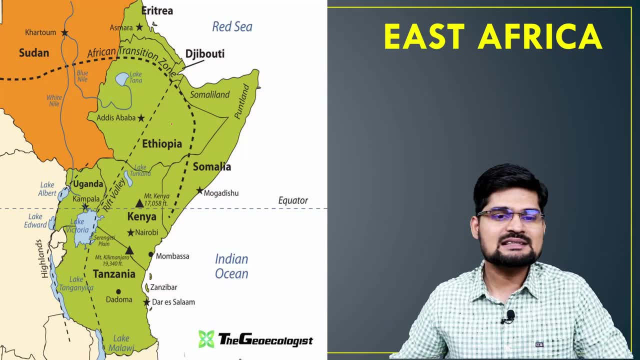 So gallancies are those people who are doing illegal mining And it is biggest problem of gold mining in terms of illegal gold mining that is happening in Ghana And they are doing illegal mining in India. So, again, these are just two例s. 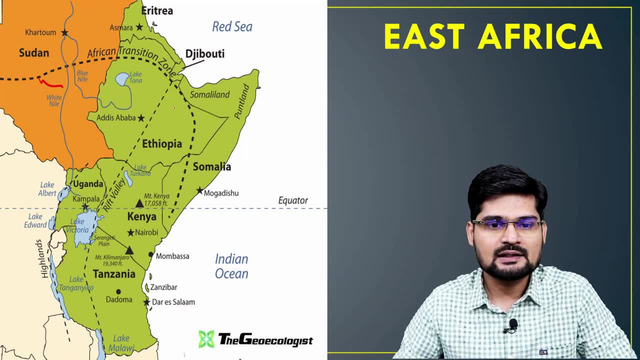 They are now doing illegal mining in South Africa. Now let us talk about the rest of the countries. So if you observe, these are the countries where you observe the East Africa. So East Africa has these countries. if you observe, Sudan is here. 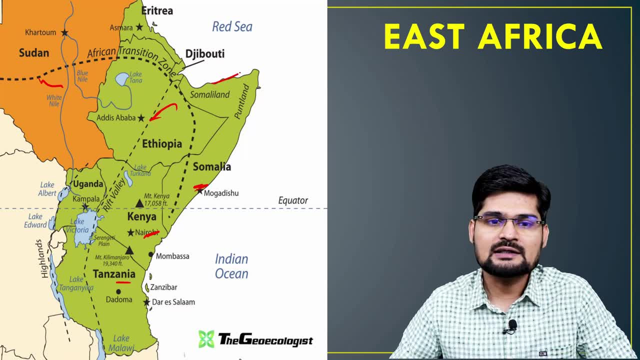 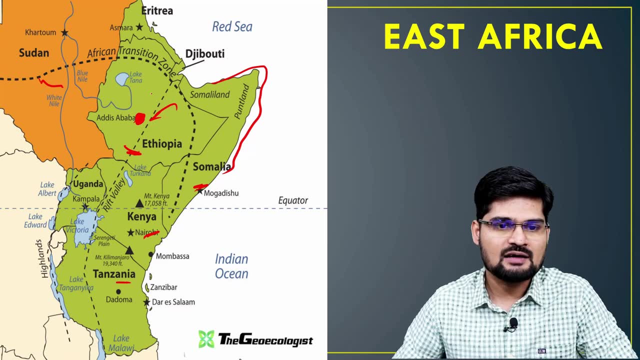 And then you have Ethiopia, Somalia, Kenya, Tanzania, So great horn of Africa. we already learned in the previous lecture as well. Now let's look into Ethiopia. Capital is Addis Ababa out here. Then you have this great African Rift Valley, and this is a transition zone from Saharan. 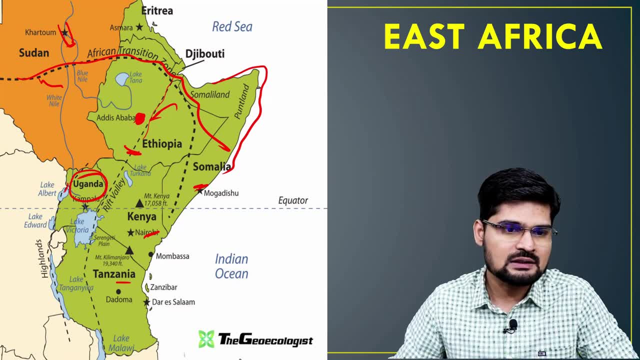 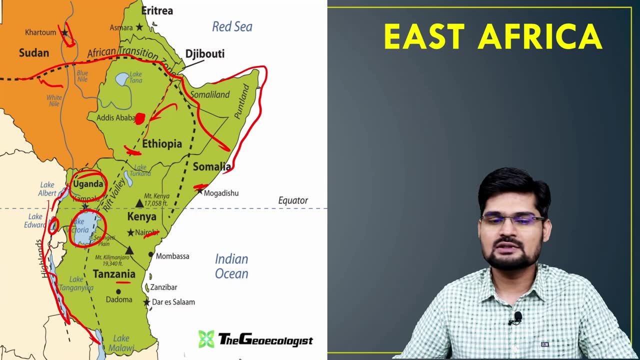 Africa to Sub-Saharan Africa, And then you have Uganda out here, Lake Alberta, Lake Edward, And then you're going further down south. You also have places like Saffron and Tic Tacs. So these are the countries, islands. so lake victoria is out here. tanzania also has this important coastline where islands 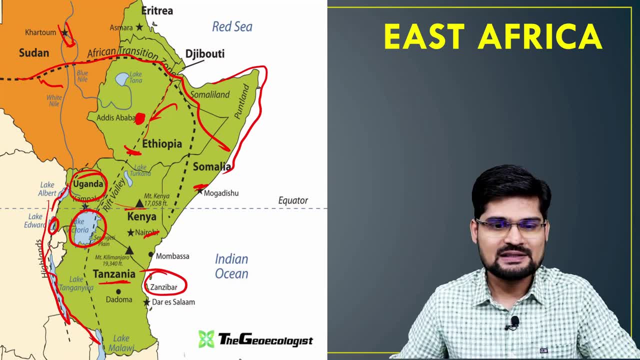 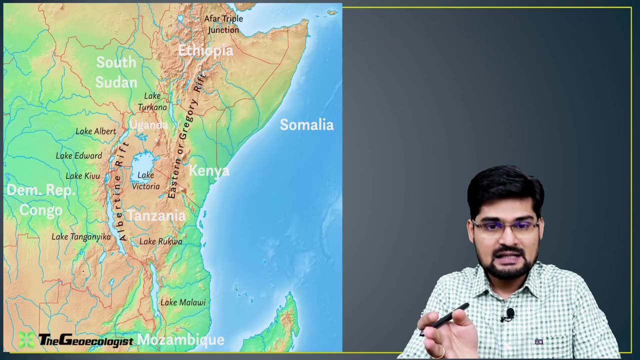 like zanzibar is there. remember island of cloves it is called, so it is found here. then kenya is a very famous country, and mount kenya is very famous out here, and mount kilimanjaro is the highest peak south of equator, as we know. so this is in tanzania, out here. so these are important places. now let's. 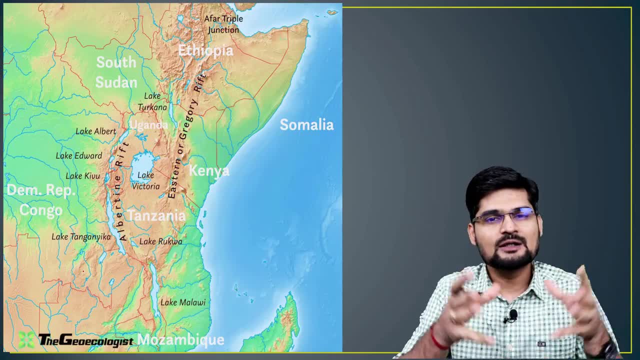 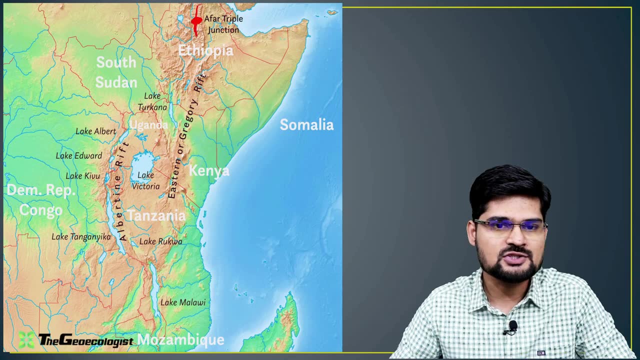 look further into the geological structure of this particular location. so what do you find? the great african rift valley, if you observe, right from ethiopia, this afar triple junction to this location, so you have this particular eastern and western rift valleys, if you observe. so this is. 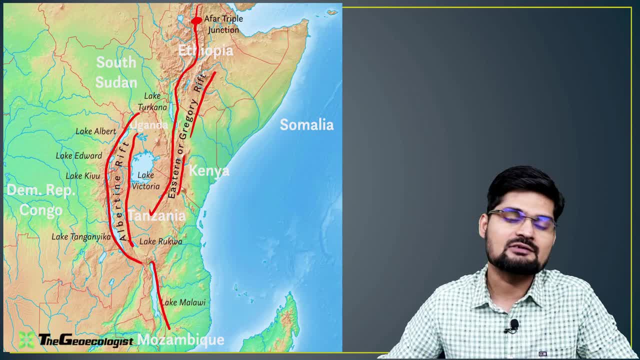 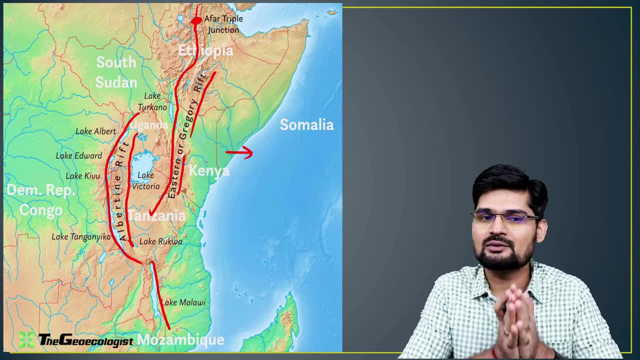 eastern, on gregory rift and this is the albertine rift. so these rift valleys are formed and this plate is in future, going to break away from the mainland africa that is being talked about right. so, if you observe carefully, so lake albert, lake edward, lake kivu, lake tanganyaka, lake rukawa. 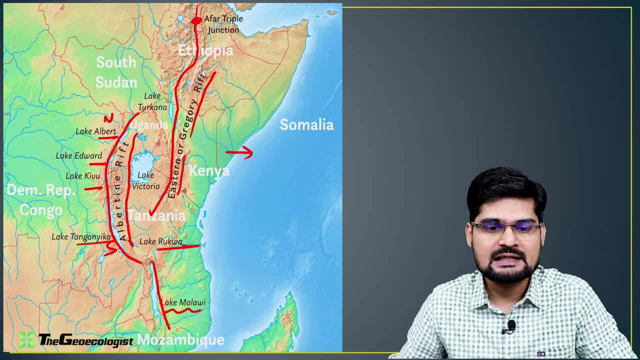 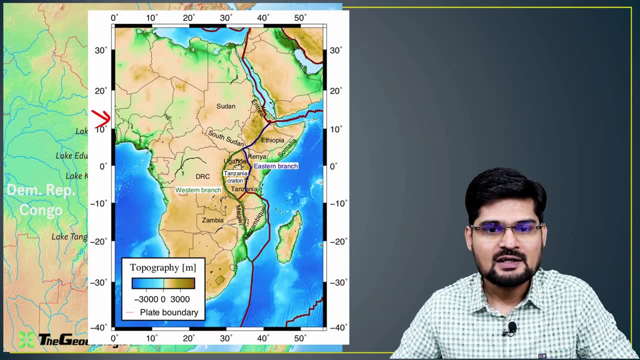 this is from north to south, and then the southernmost is lake malawi. to look further in the details, if you observe, this is one more map that will give you a clear picture of the african rift valley. so here is etria, here this particular arabian peninsula, this particular plate, arabian plate. then you have 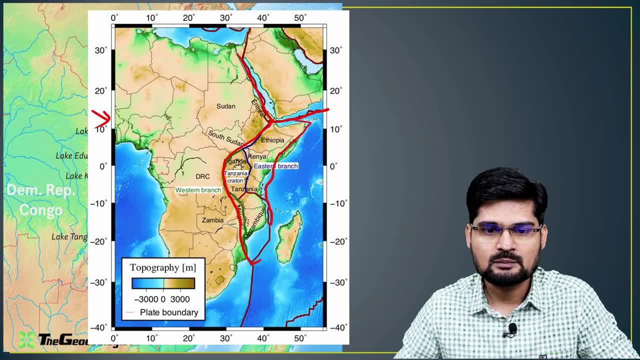 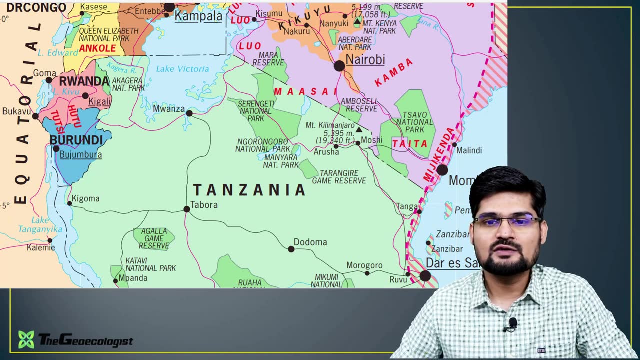 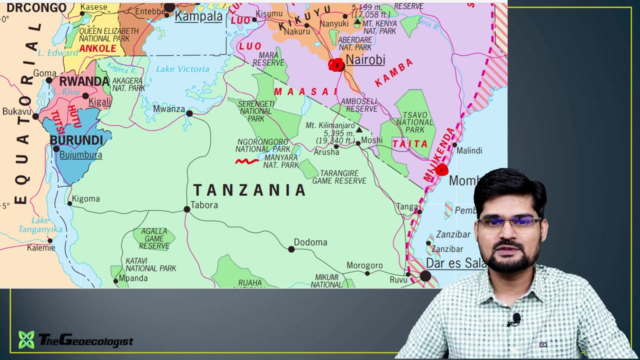 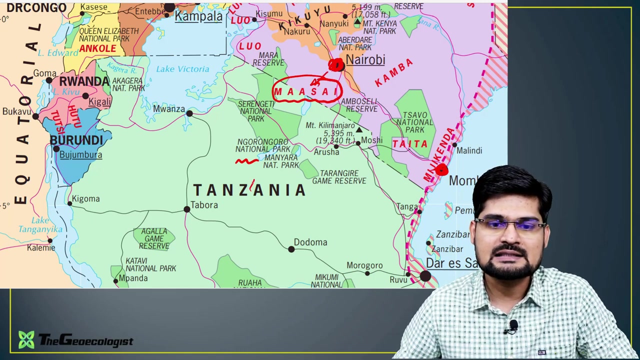 this particular kenyan side, this particular somalian plate, and then this is the african. so here is a triple junction and this is the rift valley. the tanzania craton is in between. here now we are going to look into the areas under this particular tanzania and kenya. so you remember, nairobi is here, then further mumbasa is out here, and tanzania has lot of national parks if you observe carefully. so one of the major areas is this: masai mara- remember masai tribes near nairobi, down south, and this is sharing the border of kenya and tanzania, so masai tribes. then you have serengeti national park out here, mainara national park and several other national parks in the country that you can clearly observe. so this particular area is under this particular tanzania and kenya. so you remember, nairobi is here, then further mumbasa is out here, and tanzania has lot of national parks if you observe carefully. so one of the major areas is this: masai mara- remember masai tribes near nairobi, down south, and this is sharing the border of kenya and tanzania, so masai tribes. then you have serengeti national park out here, mainara national park and several other national parks in the country that you can. 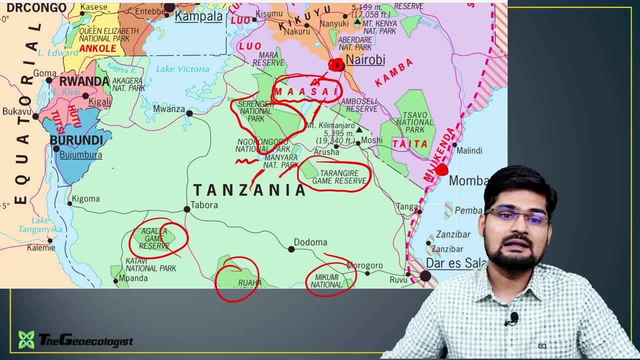 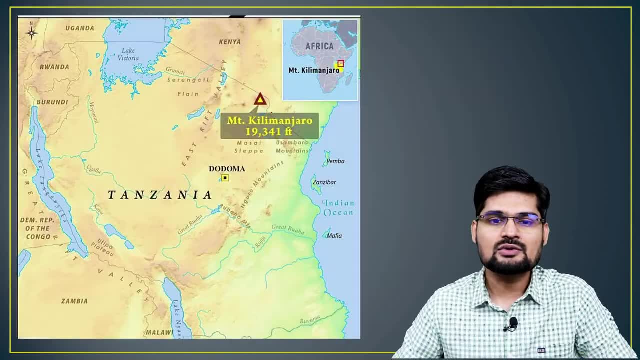 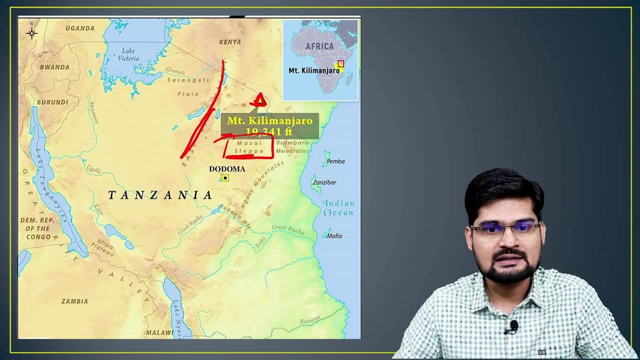 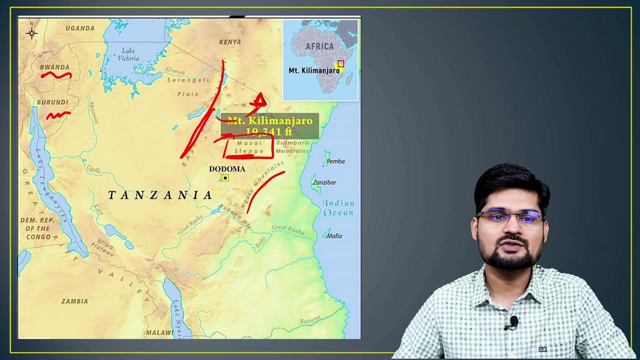 this area is rich in biodiversity, as you observed, and lake victoria serves as one of the major, biggest lake in the region, very important. and then let's look into the mount kilimanjaro. here again, this is the biggest, and here you have masai, steppe, grassland, east african rift valley and just nearby this is the highland, you have new grew mountains and it has attachment with the smaller countries in the west, rwanda and burundi. so out here in the western part now, if you further observe nairobi, that is very 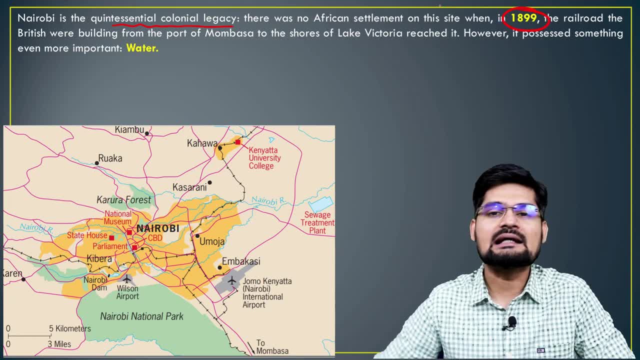 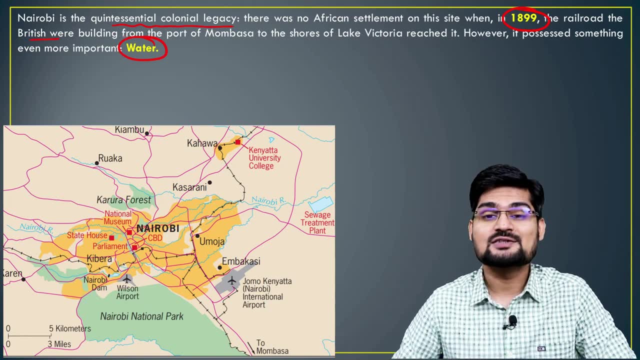 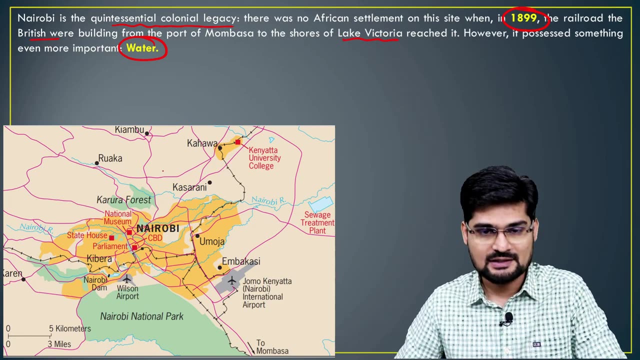 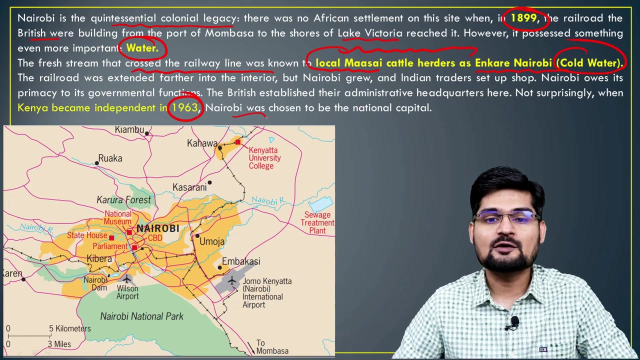 importantly, a colonial legacy, and in 1899 the rail and road was constructed by british and only because of the reason that it had a lot of fresh water. so that's how the lake victoria served as a major point for the settlement in the region, the modern settlement in the region. otherwise it was majorly inhabited by the masai and other tribes. and kenya became independent in 1963. nairobi was chosen as the national capital. so, if you observe, nairobi is obviously the primate city of this region. 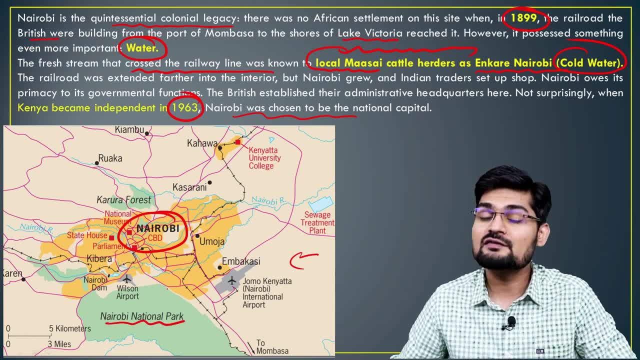 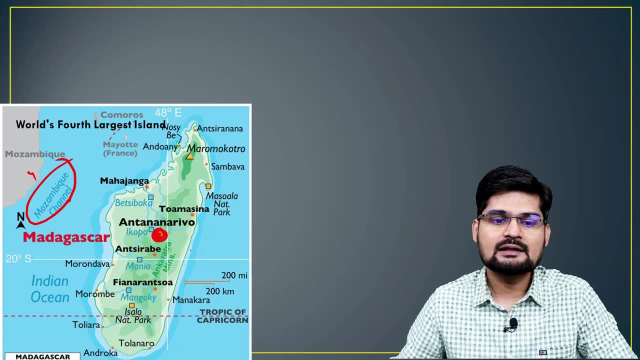 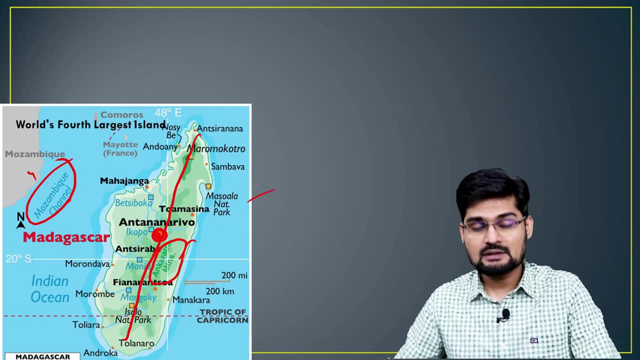 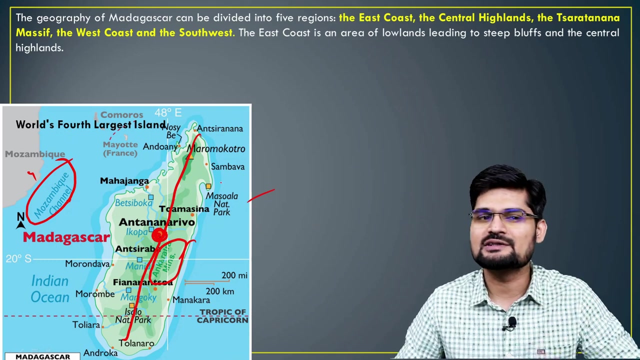 biggest city, right, and it has also a nairobi national park which is a tourist attraction. now let's go to the island that is madagascar. antona narivo is the capital out here, if you observe, and it also has the mountains, or highlands, if you observe, running from north to south across this country. and remember this area is separated from the gondwana land. 88 million years ago, by the end of almost cretaceous, it got separated and because of the separation it has a landmass which has very unique. 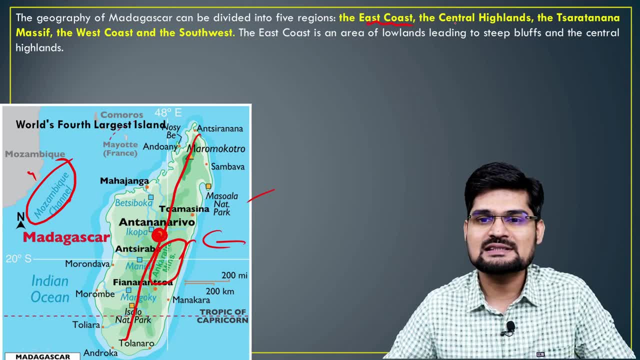 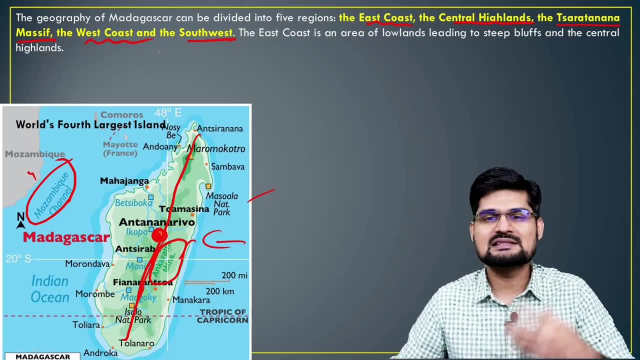 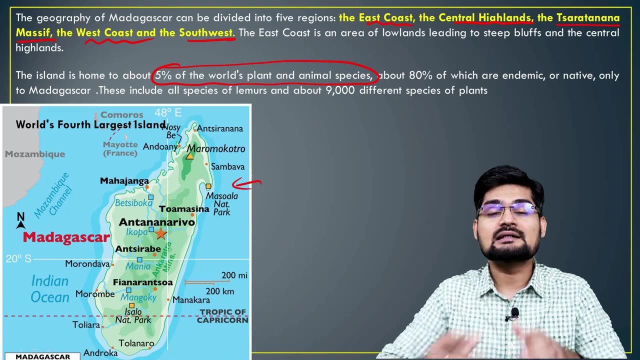 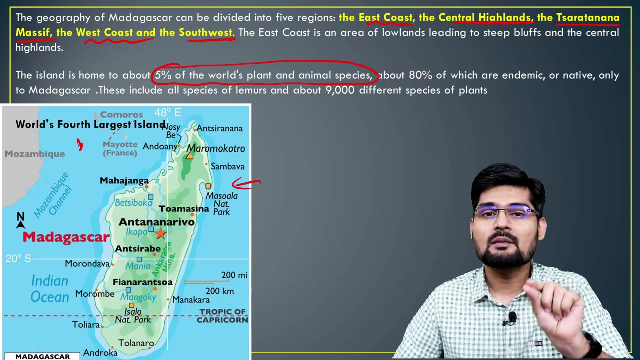 flora and fauna. so the country can be divided into east coast, central highlands, sartanana massive- that is, the central massive out here, the sartana massive- and then west coast and southwest. so this is the physical division here. but what is more striking here is that five percent of world plant and animal species is found here in this small island. this is the fourth largest island of the world but has five percent of world biodiversity, making it a biodiversity hotspot. right, and if you observe, 80 of these species are endemic. it means that you use the island to keep the plant out of the way. it can also be an 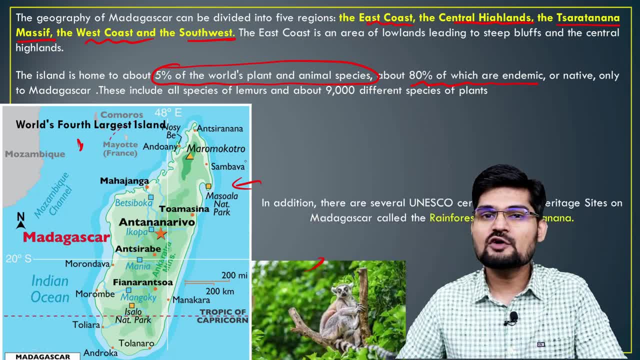 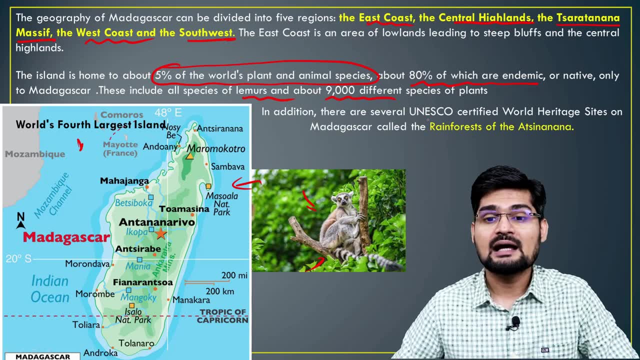 they are not found anywhere in the world. so if you observe carefully the lemurs and other 9 000 different species of plants and animals, they are only found out on this island and unesco has declared it as a world heritage site: the rainforests of astinana. so if you observe this, 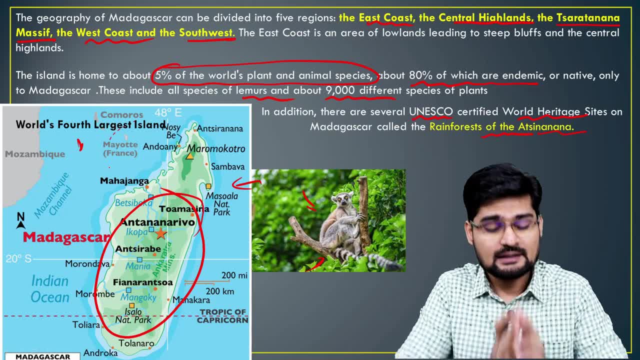 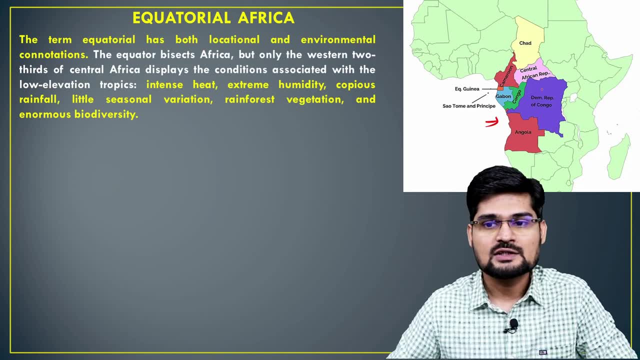 area is very much important for the world biodiversity. now, if you observe further, the equatorial africa, which has small and big countries out here connected with the atlantic coast. so right from this particular cameroon to equatorial guinea, gabon, then you have the south tome principi. 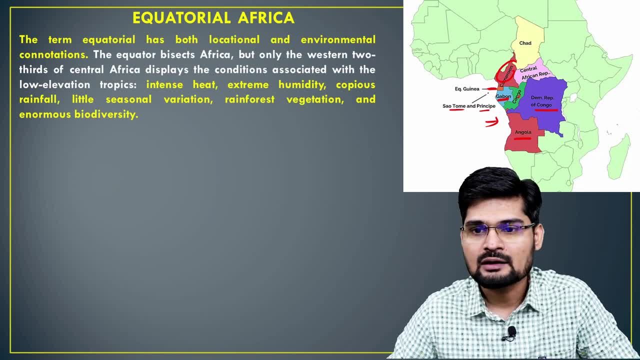 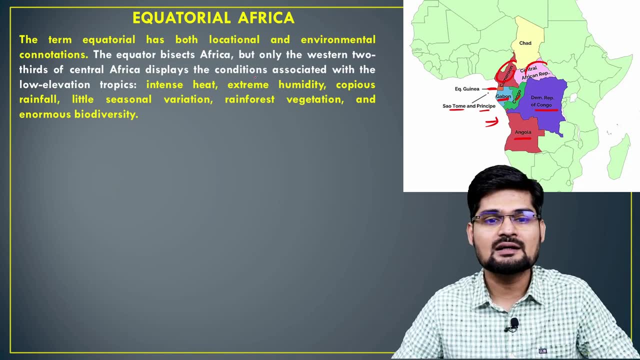 and then you have angola, then you have democratic republic of congo and congo and then central african republic. so these are on the equator and they have huge equatorial rainforests, area, steam heat, extreme humidity, copious rainfall, and also has a very little seasonal variation and rainforest. 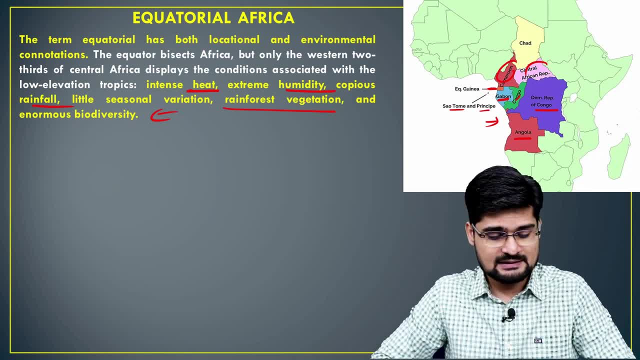 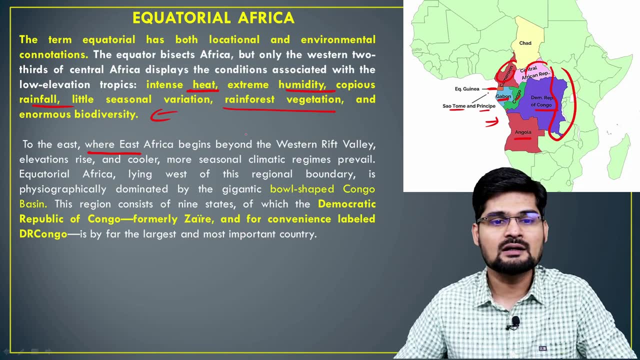 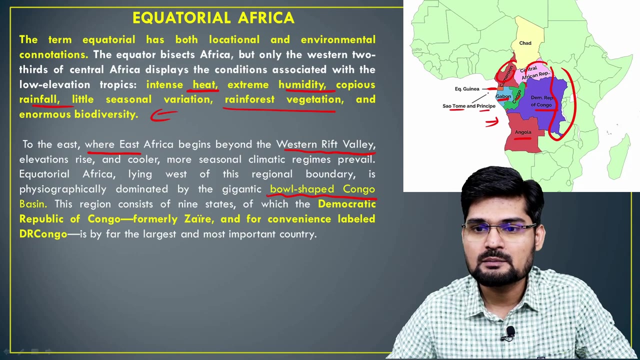 dominates equatorial rainforest, enormous biodiversity in these regions. so what is important to the east? if you go this particular site? the eastern part of this africa, that is, equatorial africa, begins beyond the west rift valley, as we can see and remember, ball-shaped congo, this particular ball-shaped 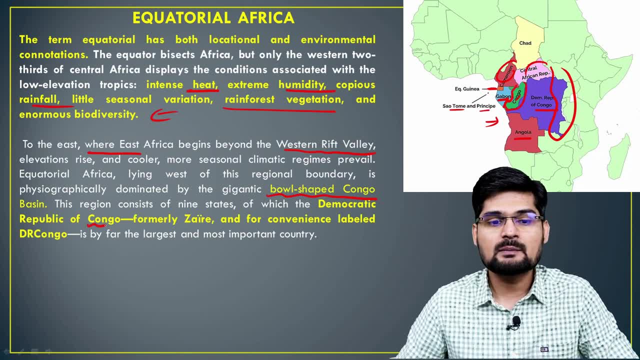 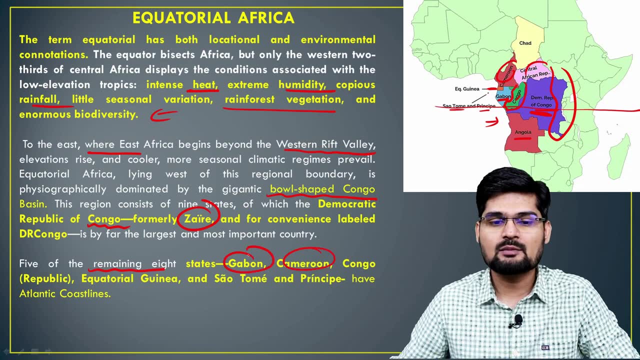 congo, if you observe, is very important here, and republic of congo. formerly it was called zaire. right, it is exactly on equator, and five of the remaining eight states, like gabon, cameron, congo, equatorial guinea, south tome and principi, they have these coastlines which are important for them. 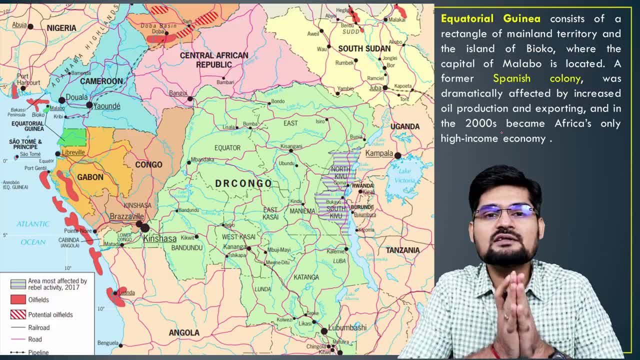 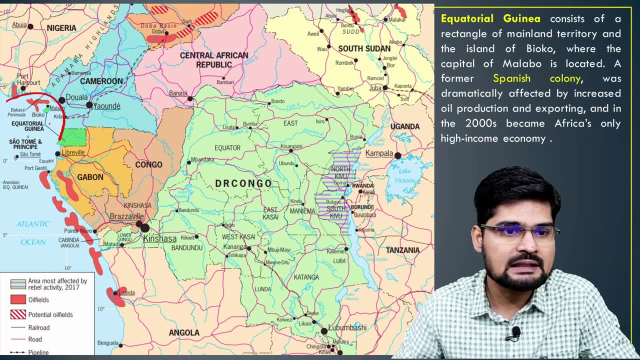 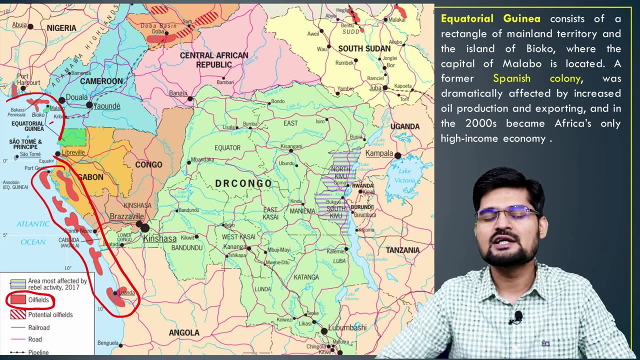 right for the economy of this country. so if you observe the details in depth of this region, you will observe carefully that this is the gulf area here- equatorial guinea- and then you will observe these red patches out here. now look at these coastal areas. these red patches are all oil fields which make the major chunk of their 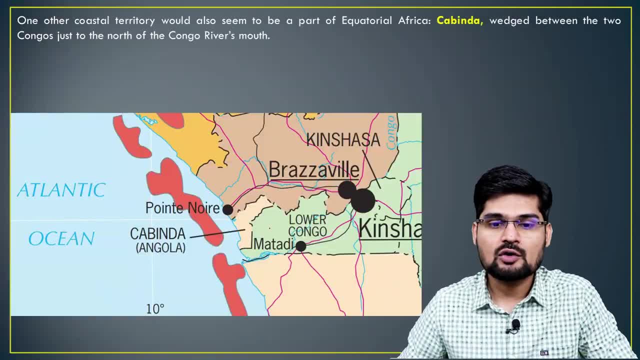 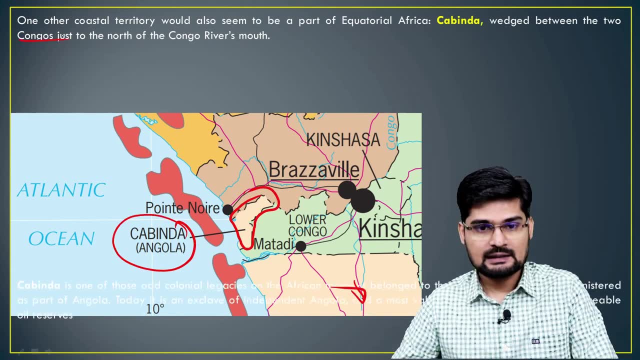 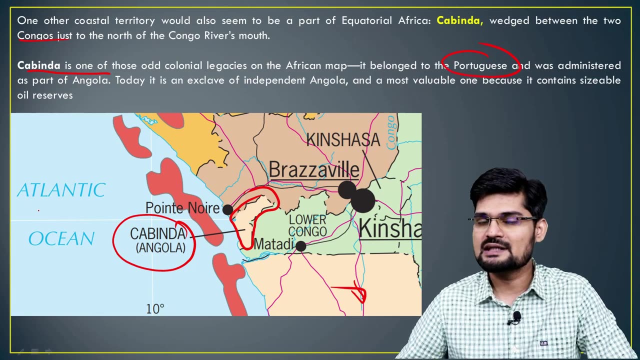 economy and when you observe carefully, between the congo and this particular area, you have this area called cabinda, which is part of the angola, which is down south. now, if you observe carefully, cabinda is one of the old colonial legacy on the african map and earlier it belonged to the portuguese and 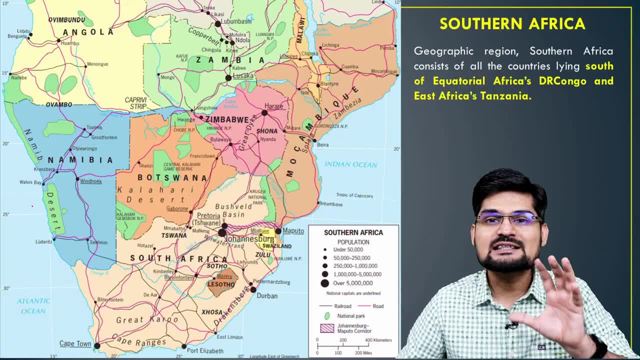 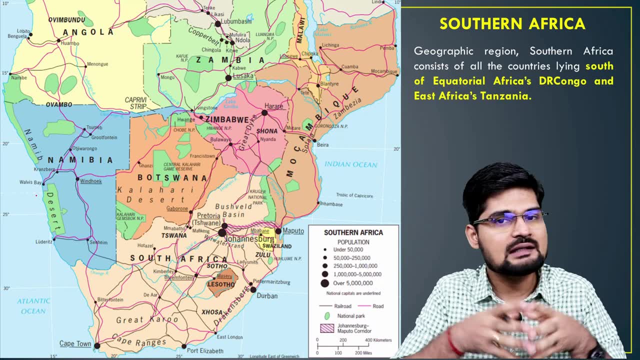 they are part of angola today. now, if you observe the southern africa and the most important area of africa that we know by the name of this southern part, the south africa and the region around it, so let's observe this particular region. so, coming down south, you have namibia. 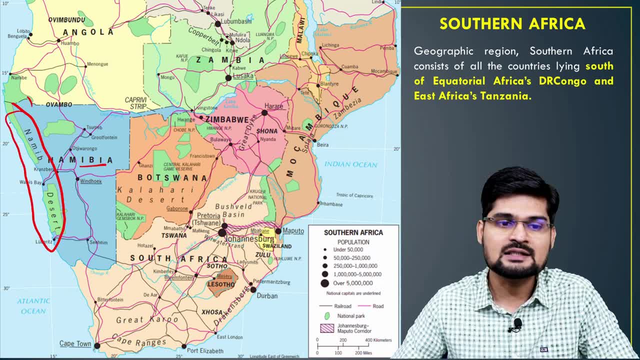 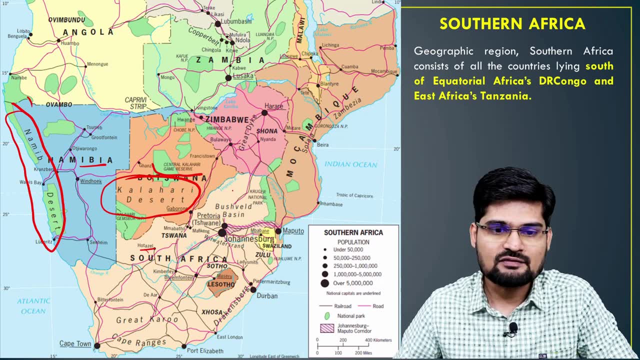 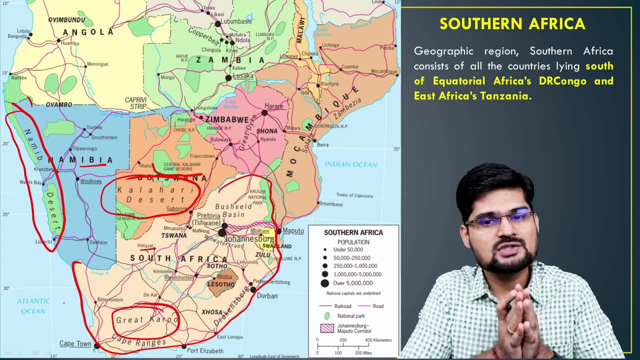 the major country and it has a major feature called namib desert, which is very important feature. then you have botswana, with the major kalahari desert- very important. then comes to the south africa, which has a highland and a coastal area country alongside the central karu region, the great karu and the small that is, a plato region, and then you will 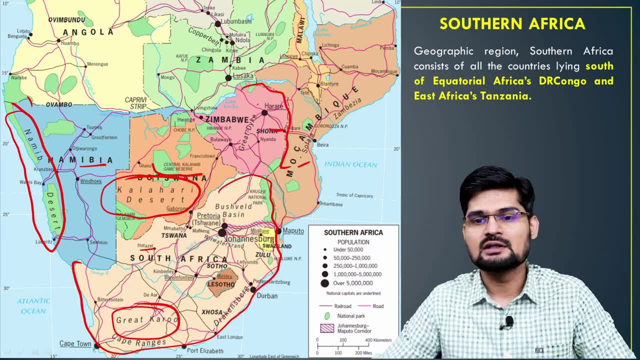 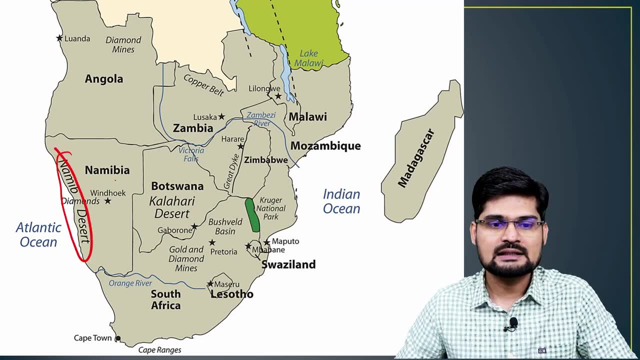 observe mozambique out here and you have zimbabwe out here. so if you observe carefully- let's look into this area- that what are the natural features? so you will observe namib deserts, then you have the kalahari desert, then you have the south africa and in between you have two enclaves, that is. 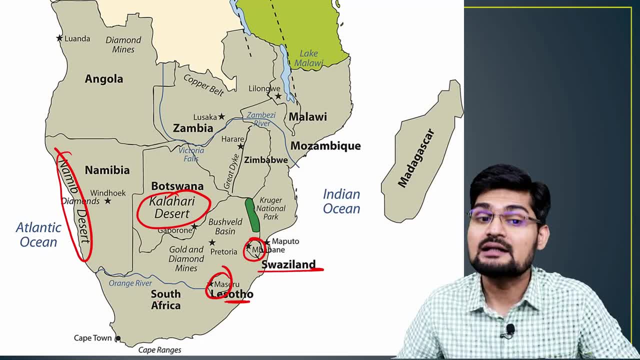 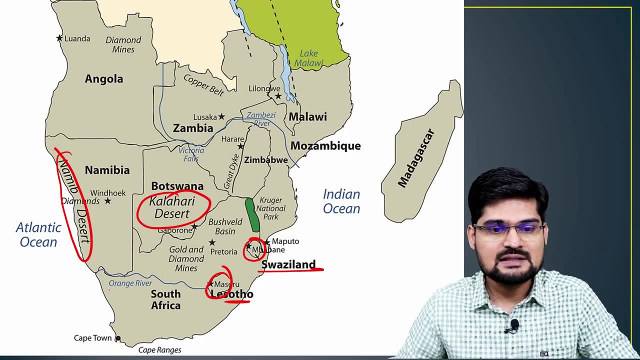 swaziland and lesotho. these are two independent countries which are inside south africa, that you say. that's why they are called enclave countries. right then you have the zambesi river in the north, you have orange river here and this limpopo river, if you. 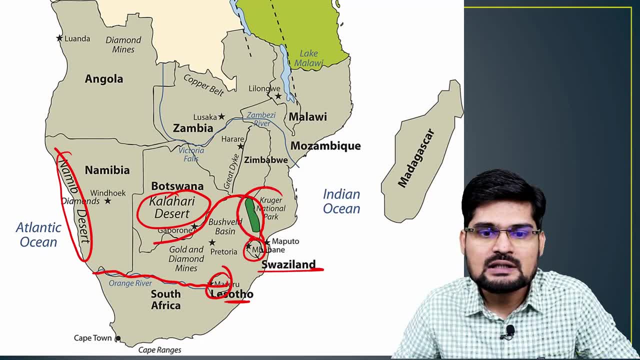 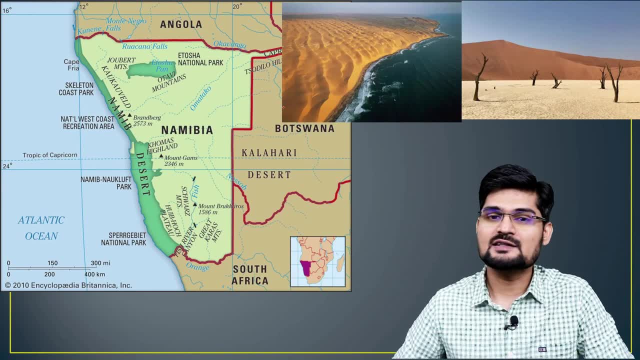 observe. this particular finds a place near kruger national park in south africa. now let's look into the further details of namibia and the namib desert, one of the very interesting areas of the world where you'll have the coastline alongside the ocean, right. so this is what 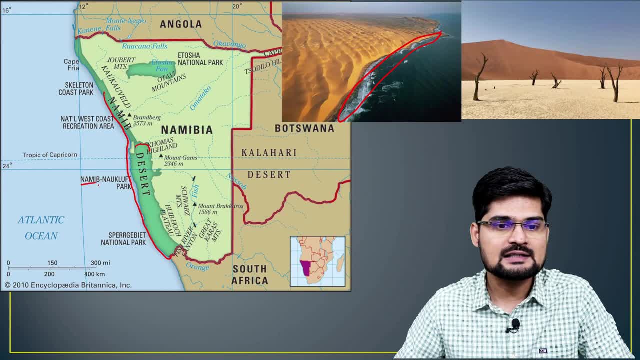 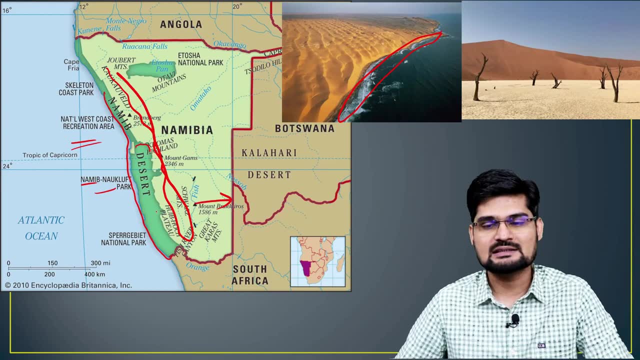 you say, is the desert, namib desert if you observe carefully. and it has the national parks as well, if you can see. and then you have the plato region and across the plato region again you have the desert conditions and not just that very interesting feature in. 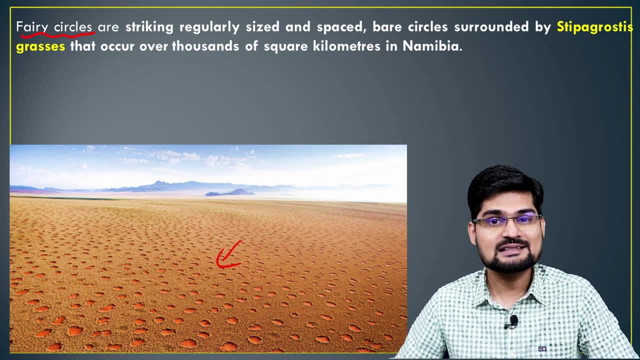 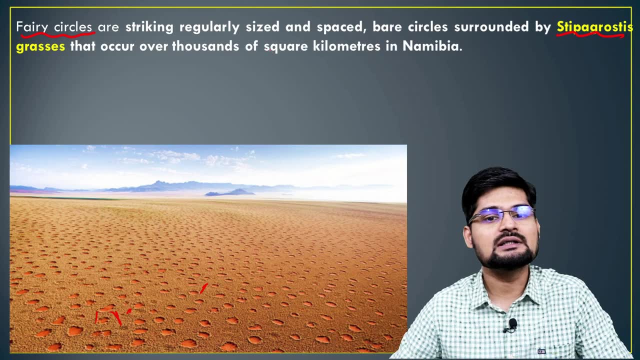 namib desert you'll find is the fairy circles which were once considered that aliens have landed here. but it's not actually like that. remember the steeper grosses grasses which are grown out here. they occur for thousands of kilometers in namibia and they are inhabited by 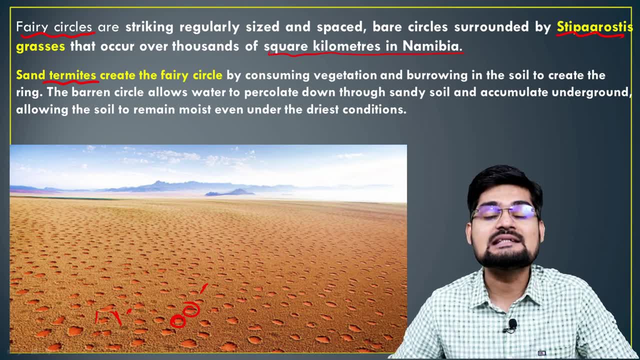 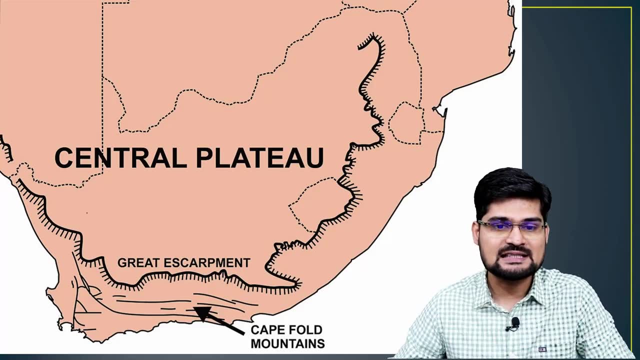 sand termites, which create these fairy circles when they eat these grasses. so you can see how these circles are created in namib desert. then, further, you see the south africa, where you have the central plato region and this is the escarpment. it is called the great. 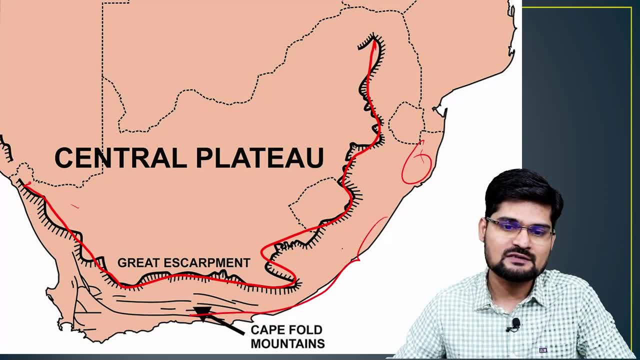 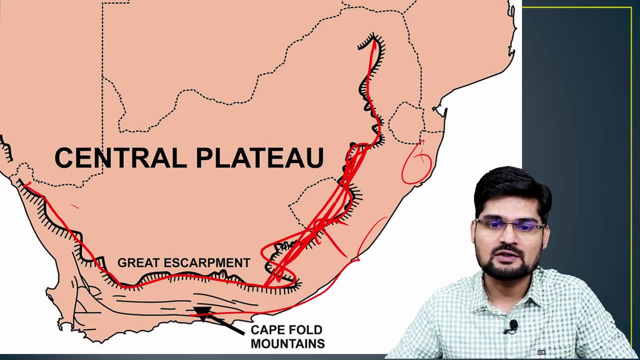 escarpment and here the coastal cities of south africa. if you observe in the background, this escarpment is visible clearly and this is the drakensberg mountain range in this particular portion out here, right. so if you observe carefully, the physical divisions of south africa, the great. 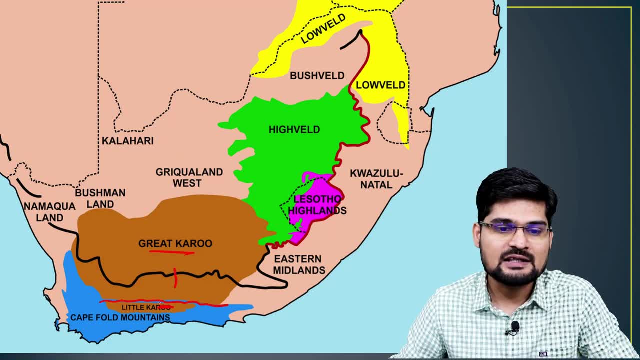 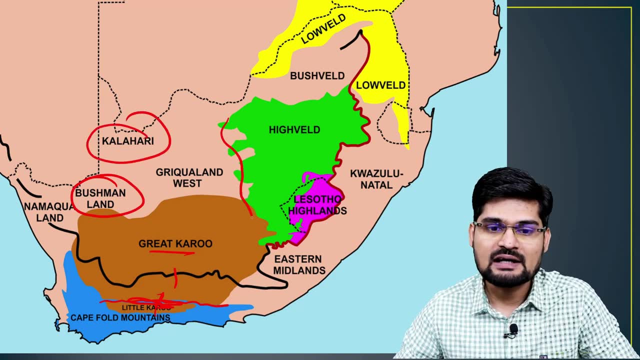 karu and little karu. in between you have the fold mountains, so this is like a valley of flood flowers between the mountains as well. here then you'll observe bushman land, then kalahari, then you have the high weld, very famous grasslands of south africa. you have bush weld, then you have low weld.